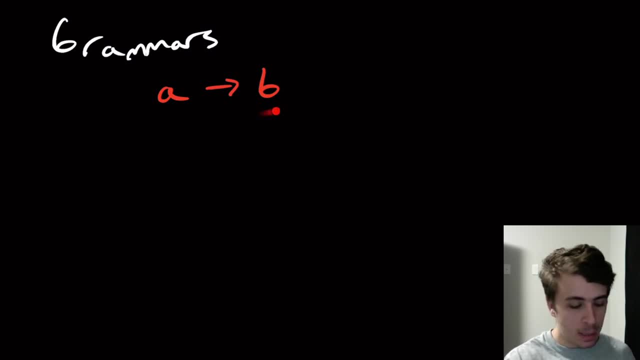 or variables, or a combination thereof, and so can B, And so that's the most general case. And then we talked about these things called regular grammars, which are which are grammars that have a particular form, which are a variable can make the empty string. a variable can make a single. 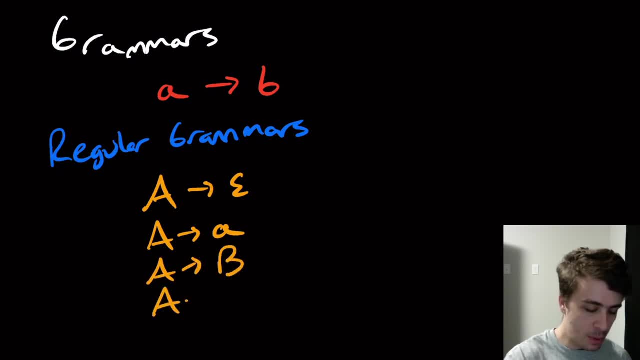 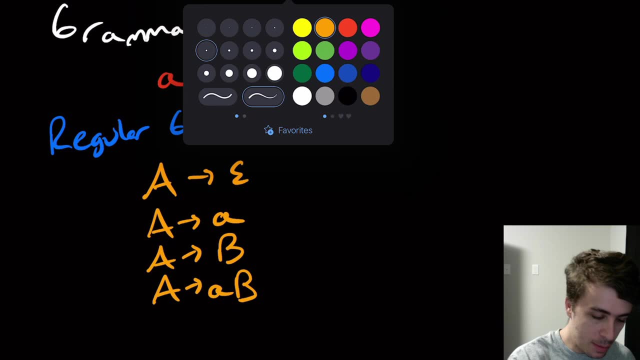 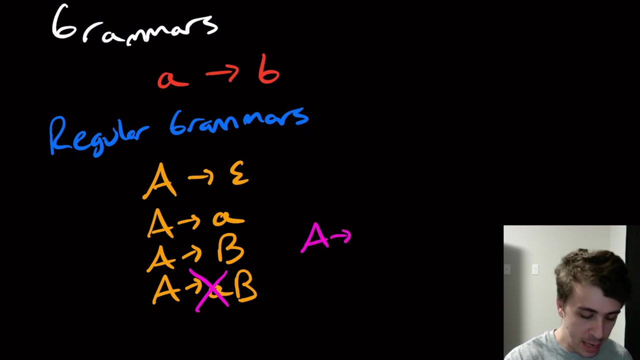 character: a variable can make another variable, or a variable can make one terminal and then a variable, in that order. I mentioned in the problem set that you can actually replace this rule right here with A goes to a variable, then the terminal. The order doesn't really matter here, You will. 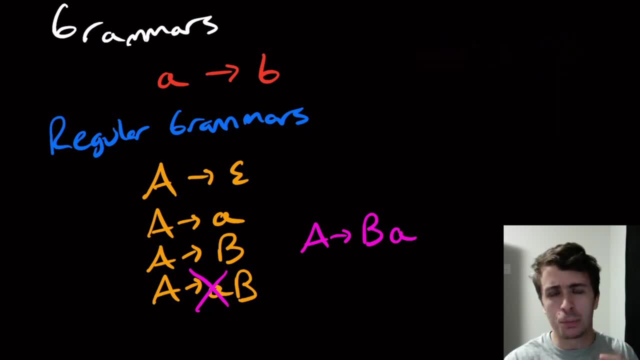 still get the regular languages. It involves proving some things about the grammar, but you still get the same things. Okay, well, what if we say I'm not gonna forbid that rule? right there, I'm going to say, yeah, I could have this type of rule and this type of rule Does. 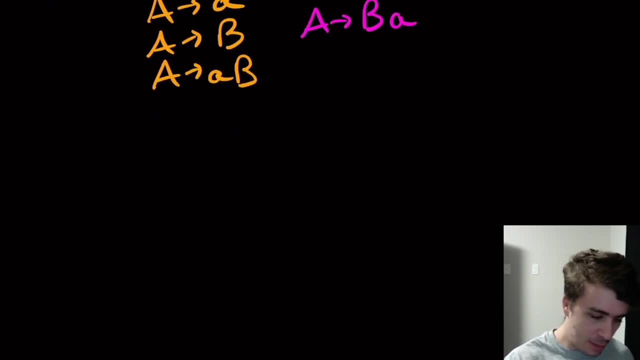 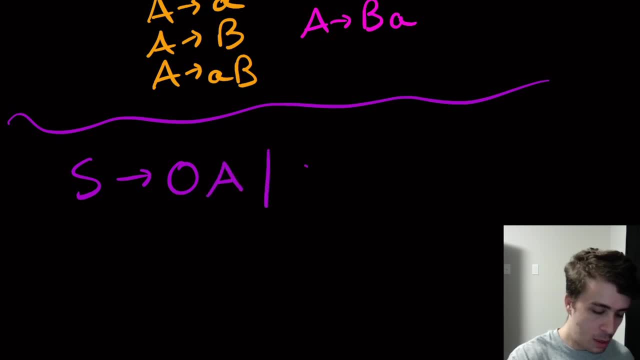 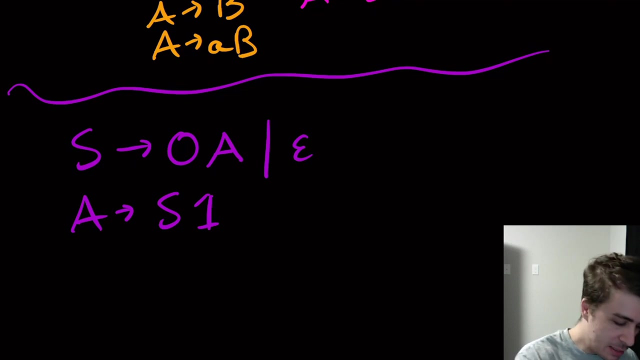 C. A is going to make zero, A or empty, and then A is going to make one wrong one. it has to be s1 in that order. Okay, so this is the grammar and s is the start variable. So this is the start variable. 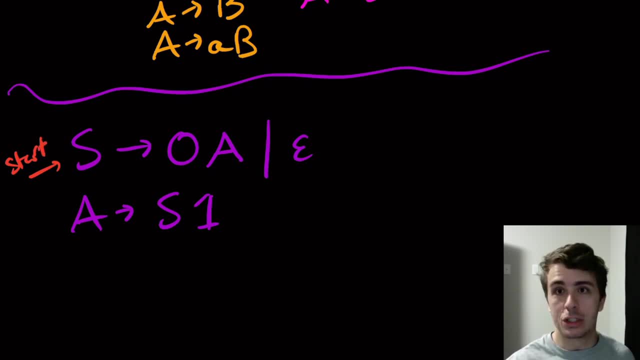 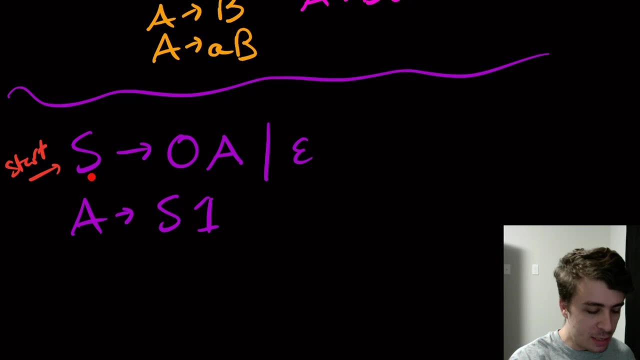 So the question is: what is the language of this grammar? So let's start and see. Well, if we look at s right here, we could make the empty strings. so let's just make a list of strings we can make, so empty we can make. what else can we make? well, if 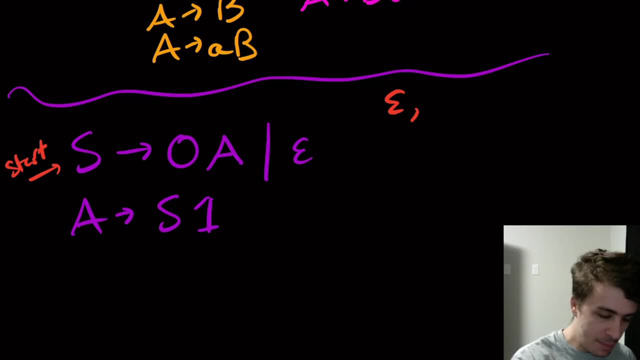 we apply the 0 to a rule, then that means we're going to have s producing 0a, because we replaced the s with the right-hand side, which is 0a. here the 0 is a terminal, by the way, and so is 1, so then we can- the only thing we can do- 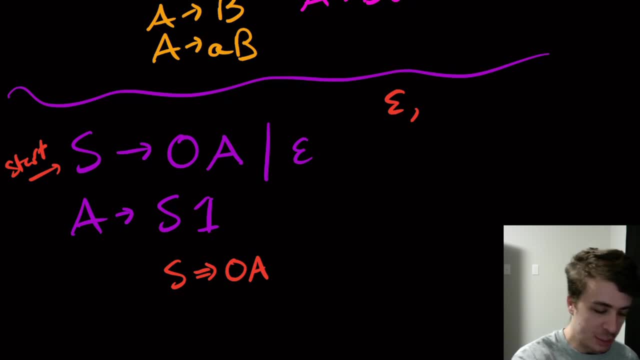 with the a variable is to replace it with s1, so therefore we're going to have 0s1 and then the same rule applies. so maybe we can replace the s with the empty string again. so that means if we replace it with the empty string, we get. 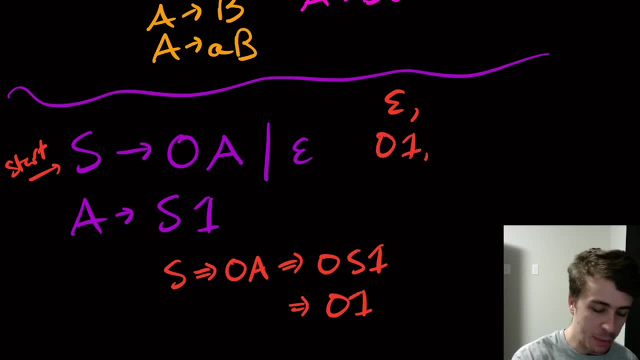 0, 1 there. so the other string, another string, we can get a 0, 1 and if we notice right here, this s right here we can apply the same two rules over and over, and over and over. so that means we can get 0, 0, 1, 1, 0, 0, 0, 1, 1, 1 and etc. wait, can we get any? 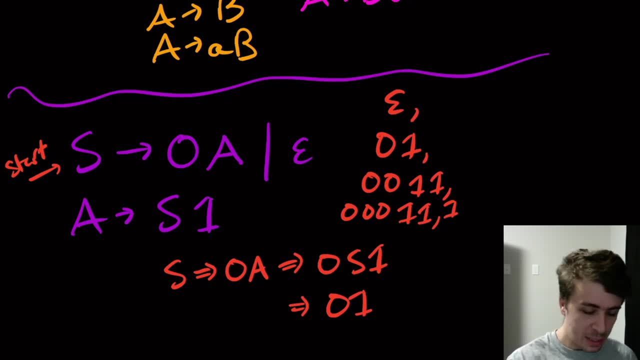 other string? well, no, because at every point any other string of terminals I mean, and I claim we can't. well, Once we have the a variable, we can only replace it with s1, because that's the only rule that's defined for it. And if we have s defined at some point, 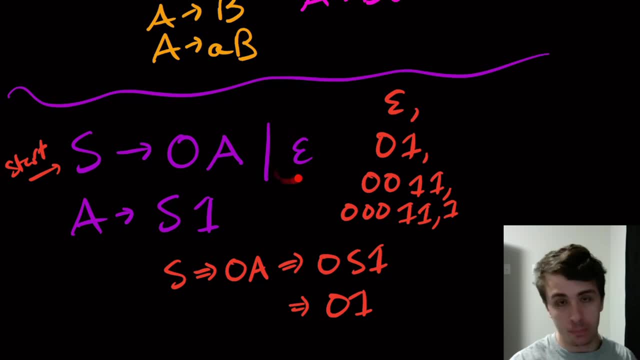 then all we can do is replace it with 0a or make it go away, And there's no rule here that replaces one variable with a rule that involves two variables. It's either that it replaces one variable and makes a variable, same thing here. 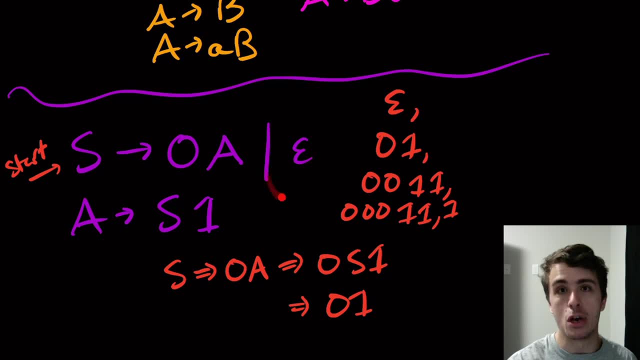 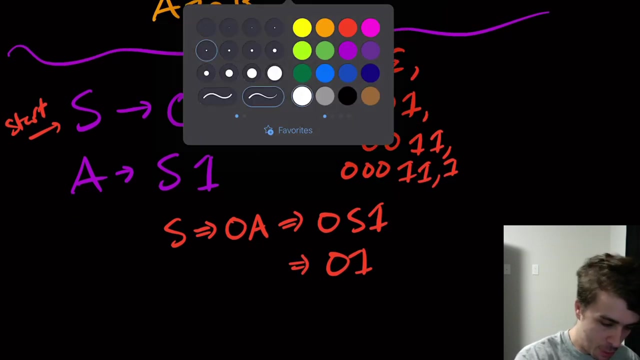 or it has one variable being replaced with no variables at all, So we always will have one variable hitching along for the ride, and then it either eventually drops out or we just keep going with one variable. So I claim then, therefore, that, given that these are the only possible strings, et cetera, 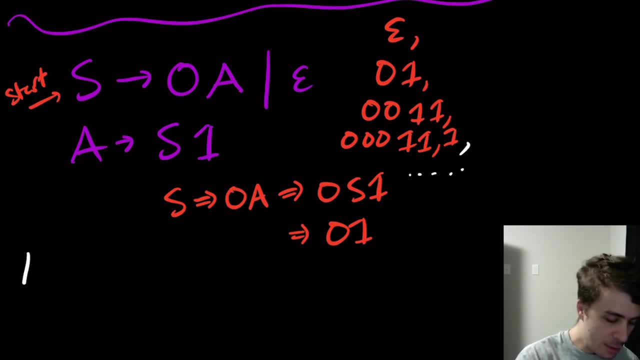 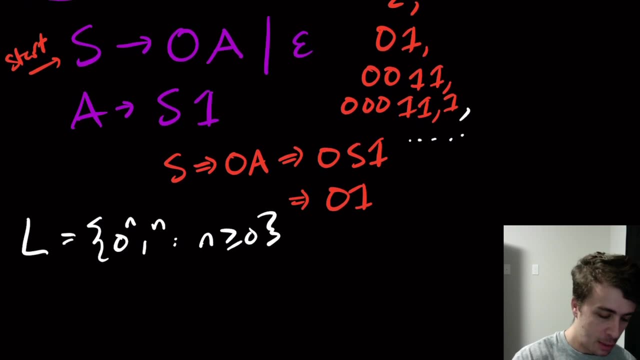 if we apply those same rules over and over, I mean, The language of this grammar is going to be 0 to the n, 1 to the n, or n is at least 0. And recall from several videos ago that this is not regular. 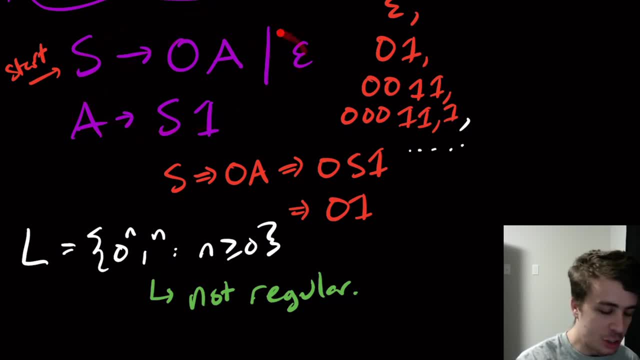 And so there are some things I should say about this. This is obviously not a regular grammar, because this says we have the definition of a regular grammar, has a term, A terminal, only on the left side, and this rule obviously breaks it. But based on this result, this tells us: 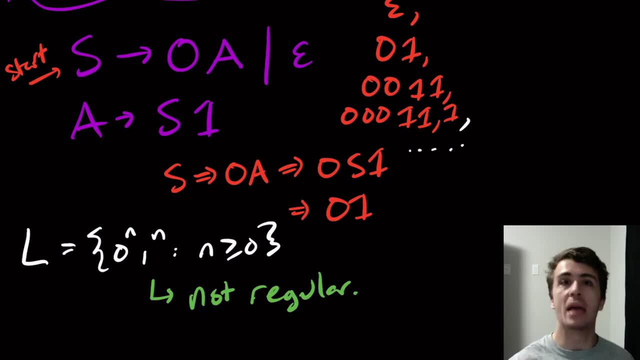 that there is no possible regular grammar you could ever create that will get this language, because regular grammars only get the regular languages to start with, And this one isn't regular. So that tells us that by changing this one, allowing that extra type of rule in there, 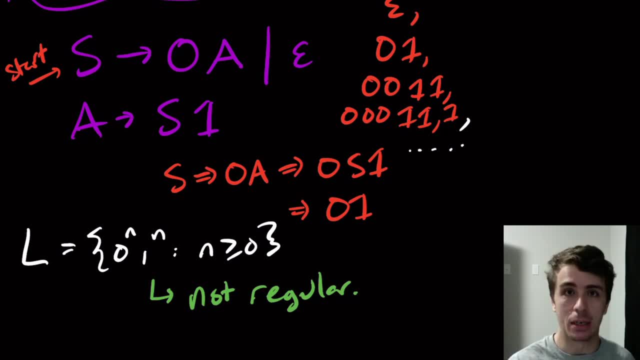 that That actually really does make a difference here. So that actually tells us something important: that the definitions that we make for certain things are really rigid in that they cannot be modified to add more stuff. But in some other cases we might be able to. 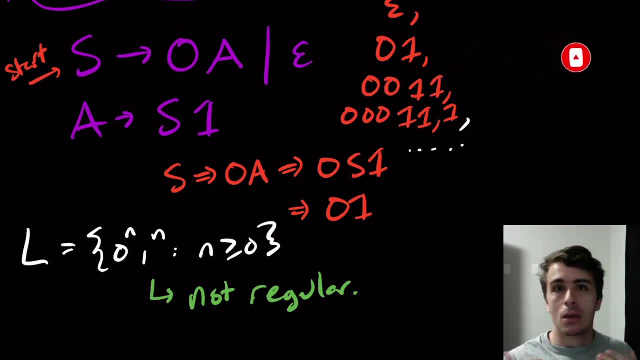 Such as when we talked about NFAs. we could have any number of final states, but we could assume that we can make an NFA with one final state by Epsilon transitioning to a single final state, And so there are some things that we can do. 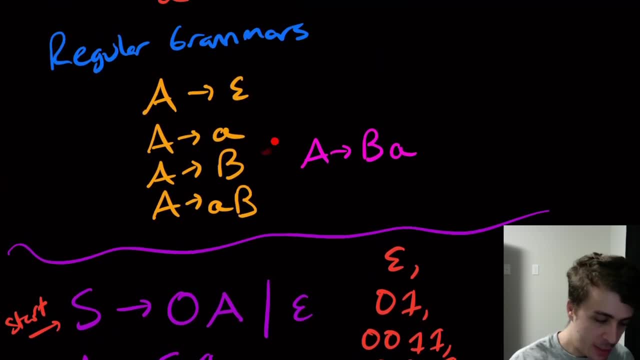 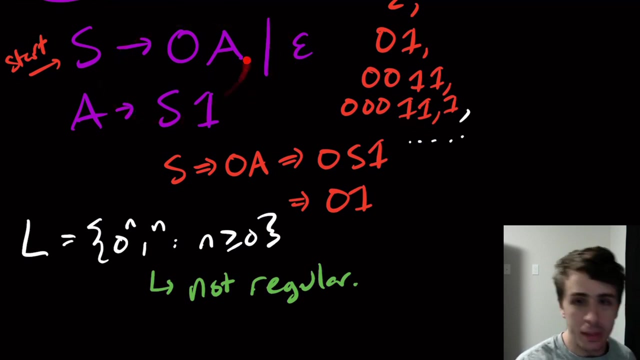 but this is an example where the definition of a regular grammar really needs to be rigid. You can either pick one of these two, but you can't pick both. OK, Bearing that in mind, well, what type of grammar should we actually call this type of thing? 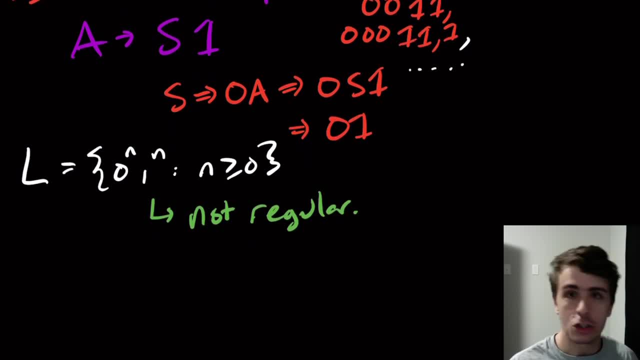 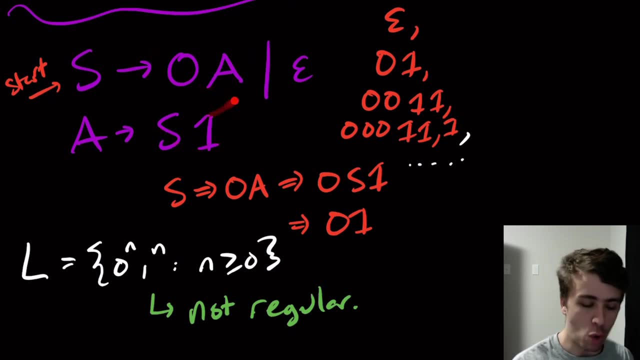 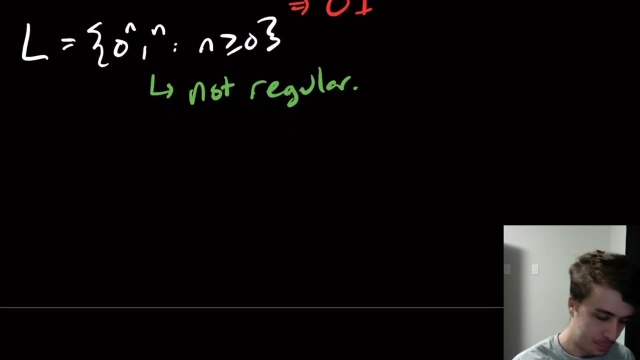 What should we even allow here? Well, let's actually just go for broke and say: you can put anything that you want on the right side. It doesn't have to be one terminal and one variable or something. You can put anything you want in any order on the right side. 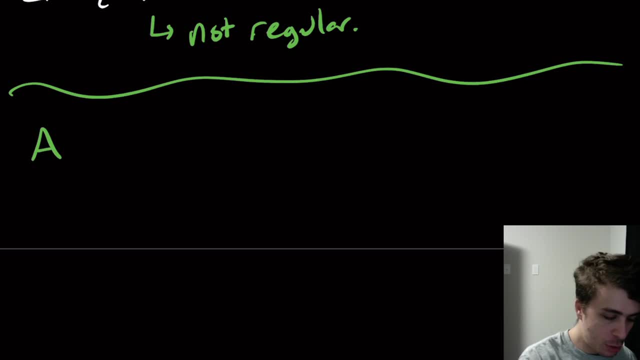 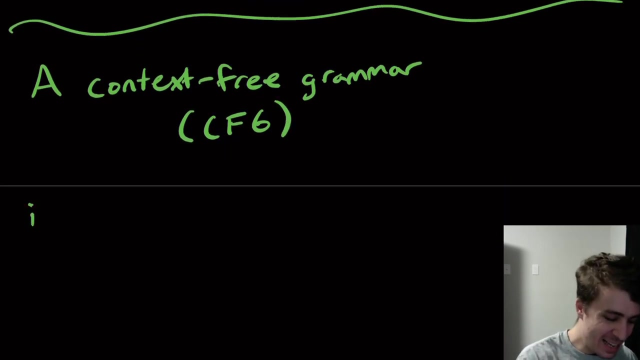 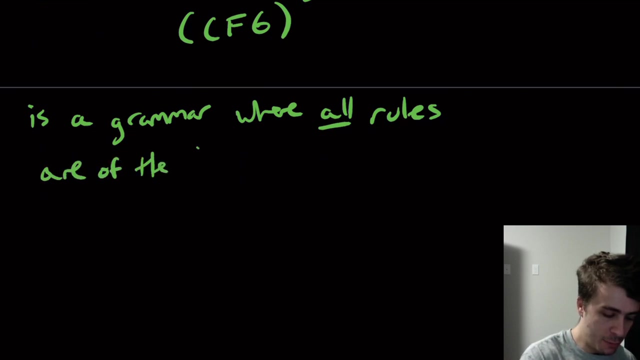 So that's what we're going to look at here, So something called a context-free grammar- and I'll explain where that comes from- which is abbreviated CFG. naturally It is. It is a grammar where all rules are of the form a goes to x. 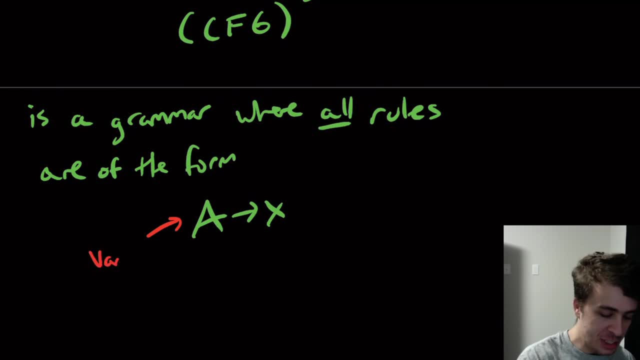 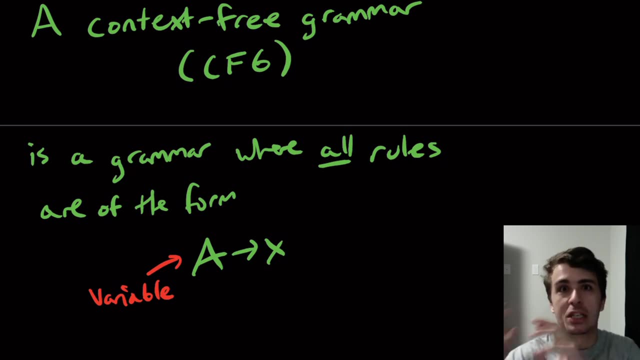 where the a right here. that's a single variable. So it's always going to have a single variable on the left side. So it's not like we're replacing multiple things with multiple things. We're always replacing one variable. no terminals at all. 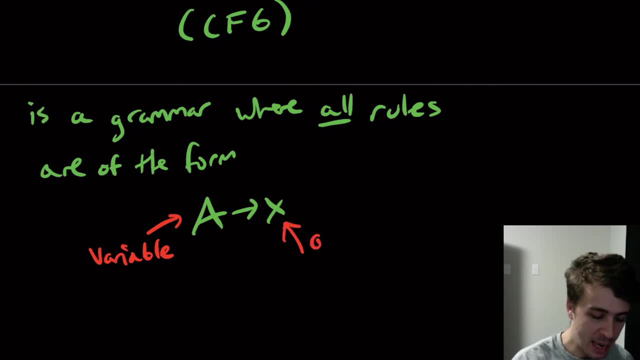 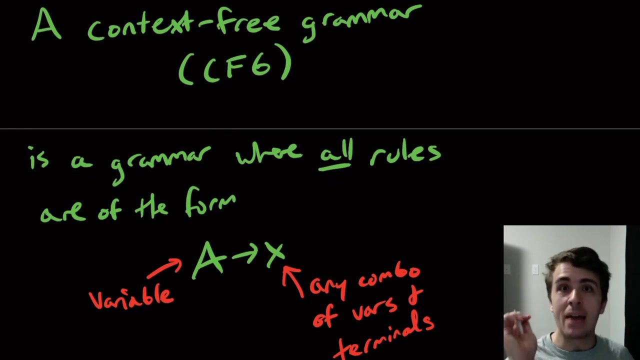 And the x on the right-hand side can be any combo of variables and terminals, any empty string, of course. So this is saying that you can have anything you want on the right-hand side. So every grammar we've ever talked about, every explicit 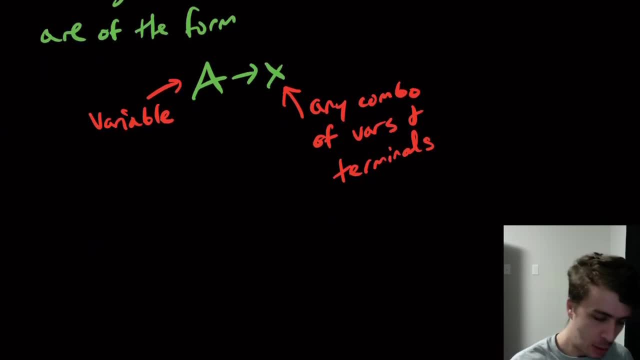 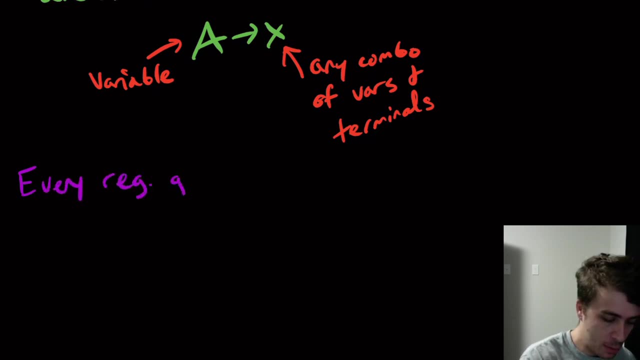 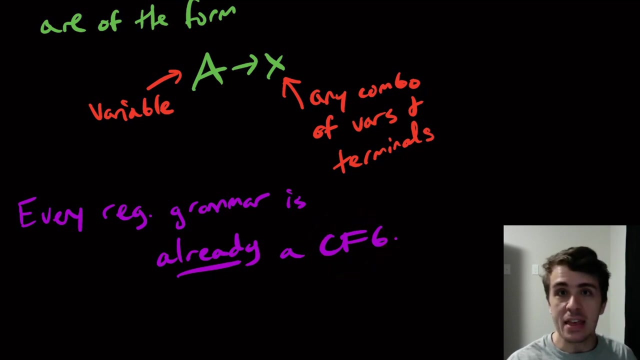 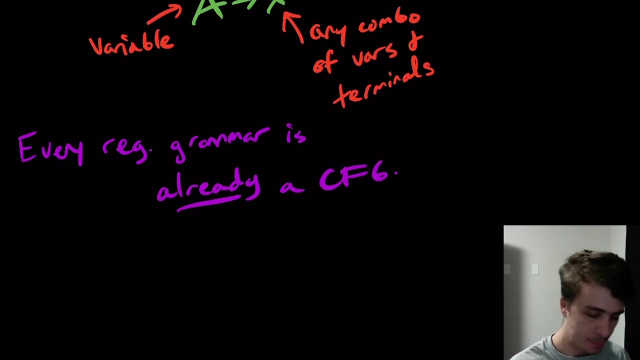 example of a grammar is already a context-free grammar. So this tells us that every regular grammar is already a CFG, because CFG says you can have anything you want on the right-hand side, whereas regular grammar restricts what you can have. So it's already a context-free grammar. 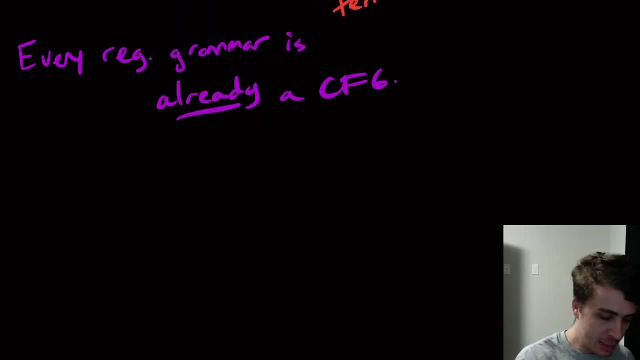 And there's one more definition, which is a context-free language, which is abbreviated CFL is the language of some CFG, So it's the analogous. So if this thing, like regular language, was for DFA, context-free language is for context-free grammar. 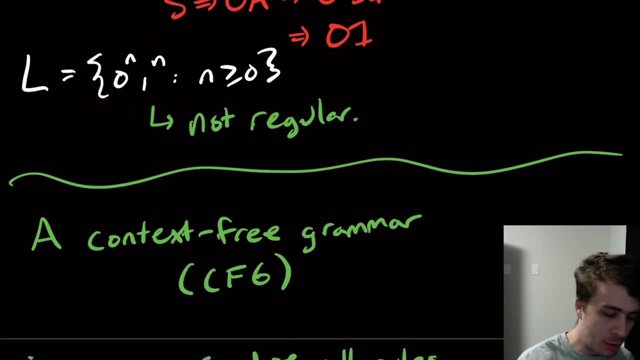 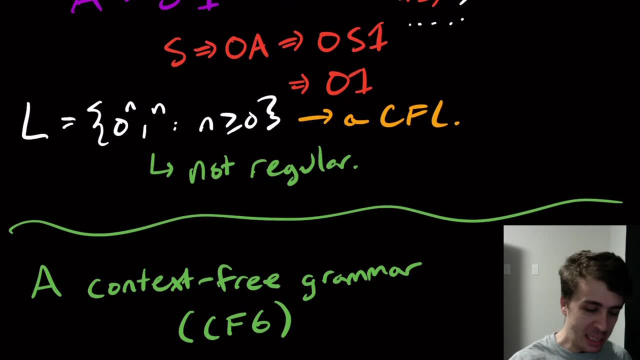 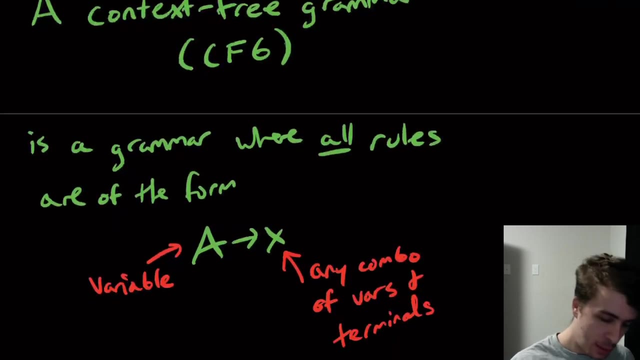 So in this case, for example, this language right here is a CFL. It's a context-free language, because I just exhibited a grammar for you, a context-free grammar for you- that has that language. And another thing we should note from this: 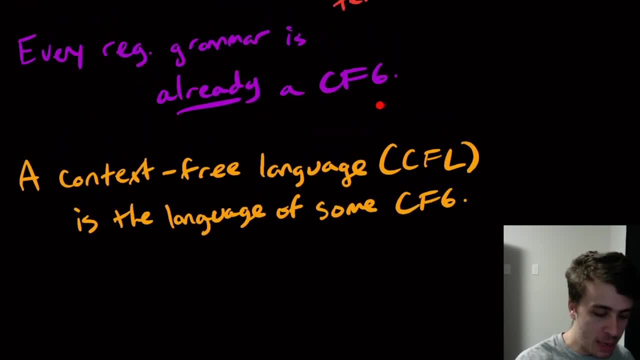 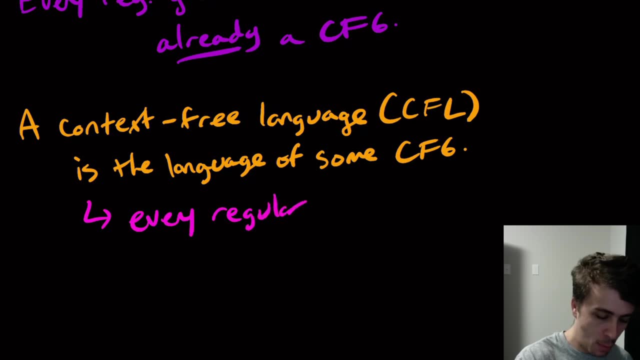 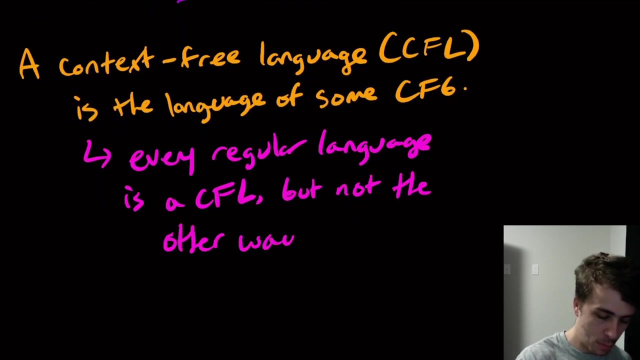 in the previous statement. right here, every regular grammar is already a context-free grammar. This tells us that every regular language is a CFL, but not the other way. Why not the other way? Because, 0 to the n, 1 to the n, that language is not regular. 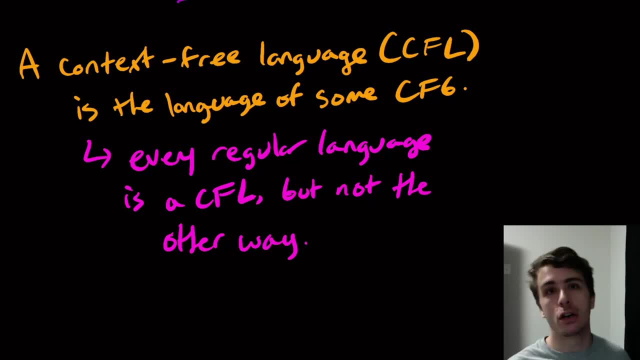 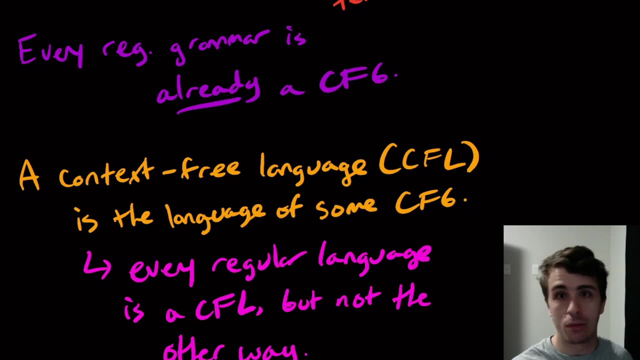 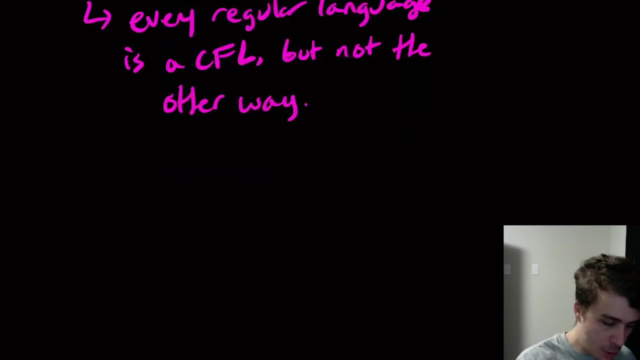 So there are some context-free languages that are not regular, but every regular language is a context-free language, because every regular grammar is a context-free grammar. OK, So let's do a quick example. So let's do this one. I call it PAL. 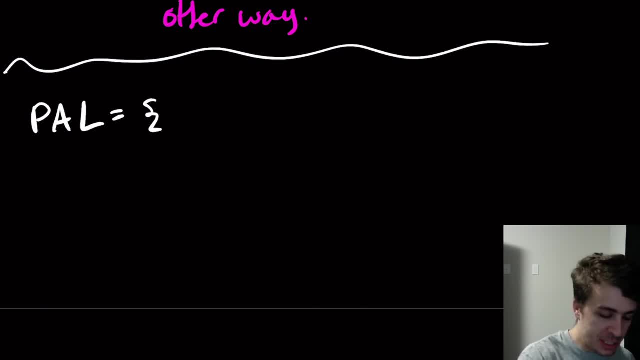 So what is this? So this is the set of all PALs. So this is 1 over a palindrome. OK, so we've got a set of all PALs here. I'm going to write a set of 5 palindromes over a 0, 1 star. 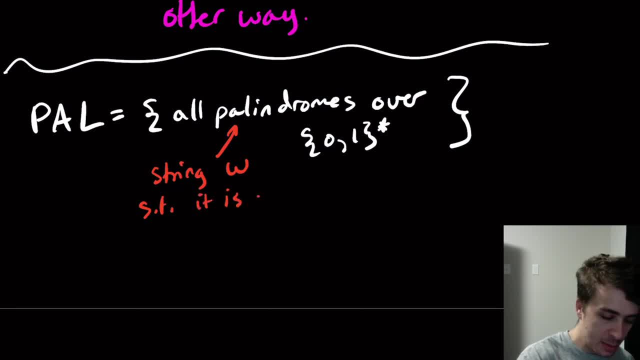 I'm going to do it this way, OK? And if you happen to not know, a palindrome is a string W, such that it is equal to its reverse. So I can read this out: This is a set of 5 palindromes. This is a set of 5 palindromes, So I can read this out. So if I want to write a set of 5 palindromes, So if I want to write a set of 5, 1 over a palindrome. 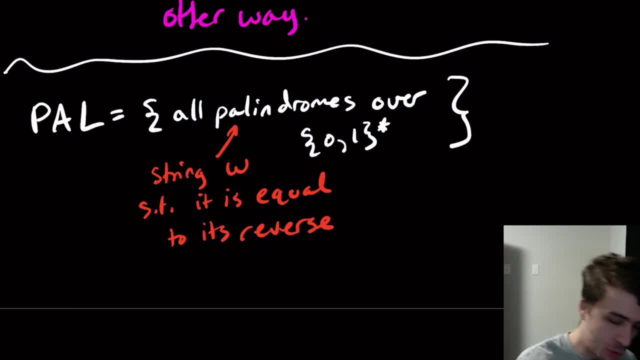 the string W backwards and forwards and it's exactly the same string. So, as an example, 0, 1, 1, 0 is a palindrome And so this string would belong in there, The empty string's in there, Individual characters are in there: 0, 1, 0, 0's in there, et cetera. So there are a lot. 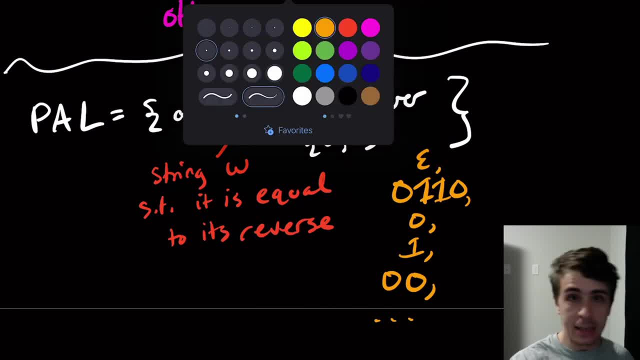 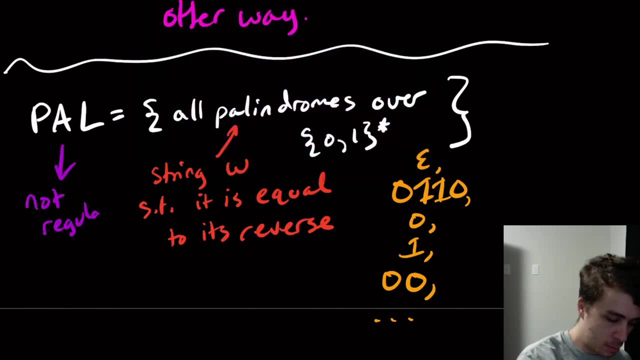 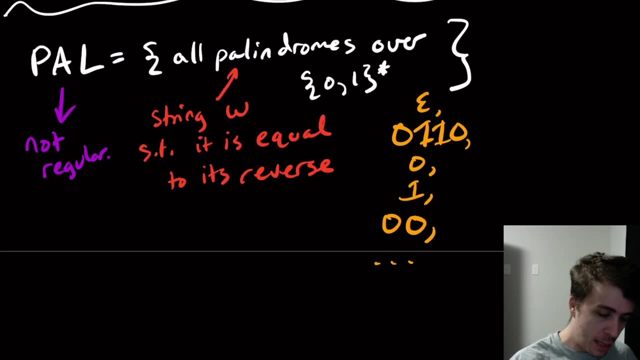 of strings in here And I claim- and I want you to be able to prove it in the comments- that this language is not regular And not really important for our purposes right now, but it is just not regular. Okay, so how do we? I claim here that pal is a context-free language. 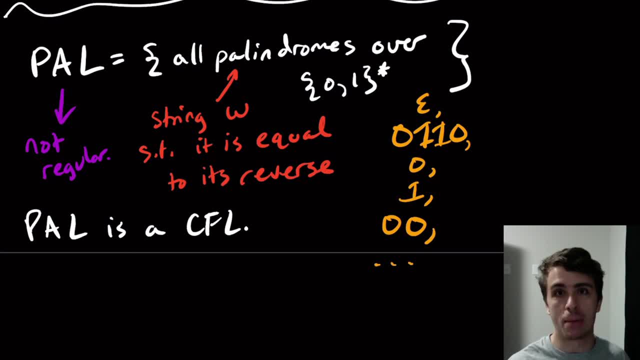 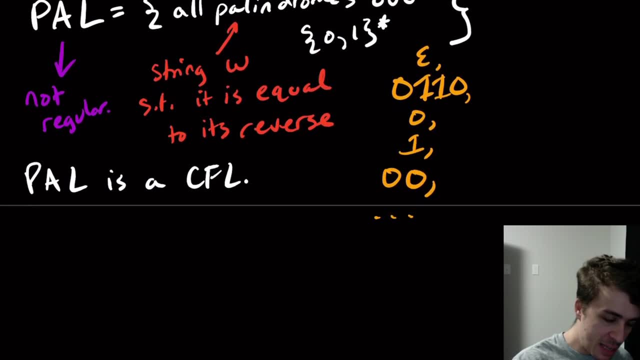 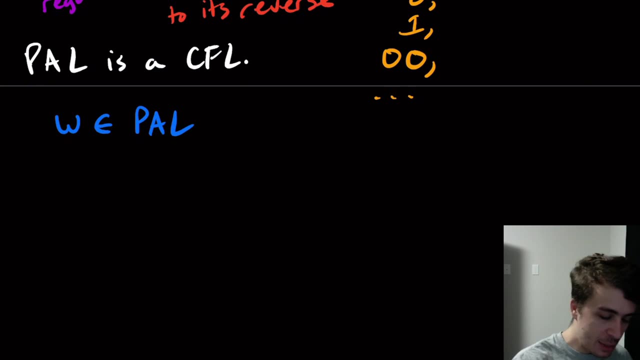 So that means that I can make a context-free grammar for you for this language. So let's actually think about what this language is. Well, let's say that W is a string in the palindrome's language. So then that means: well, it either starts with a 0 or it starts with a 1.. 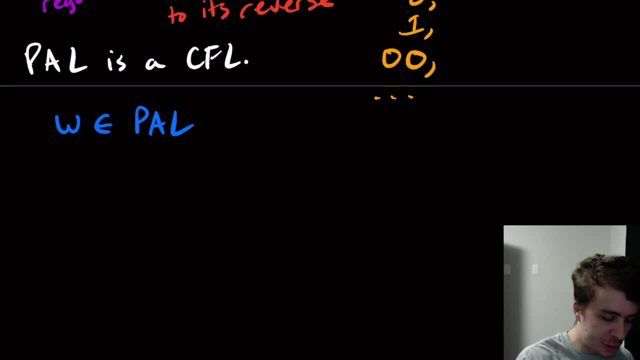 I don't know which, but it starts with one of them. So let's say it starts with a 0. Well, if it starts with a 0, then what happens is that at the other end, because it's equal to its, 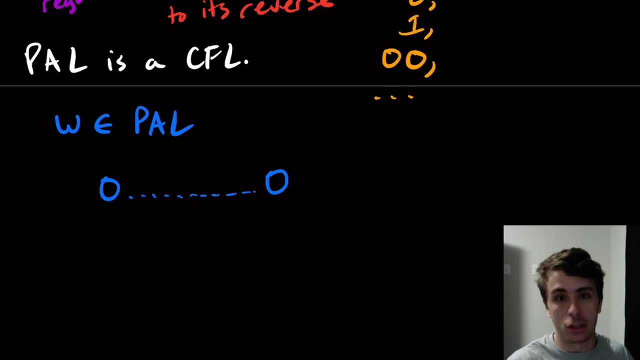 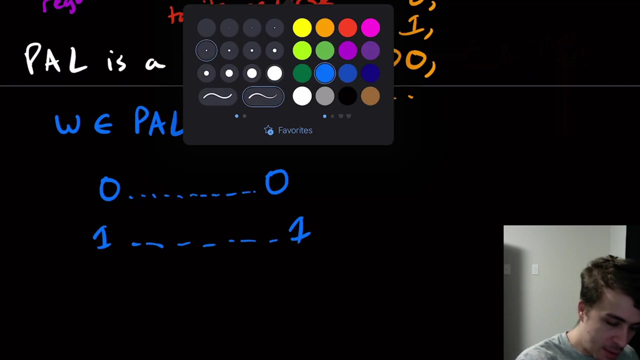 character, the last character of it. well, it even might be the same character, but the last character must also be 0, because it's the same backwards and forwards. And if it started with a 1, it's exactly the same principle. It also ends with a 1.. So, but the key here that you should 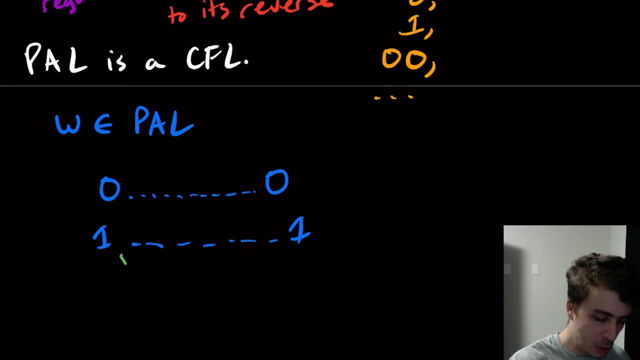 notice when you're making context-free grammars is what happens in the middle, Because the way that context-free grammars are usually made is especially important when you're making a new, very recursive-like structure, in that you try to solve a small suppose that you can solve the. 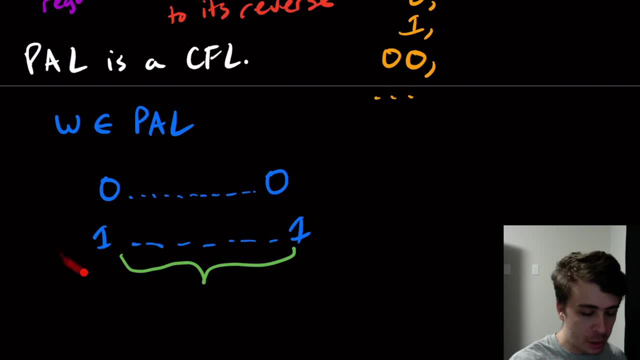 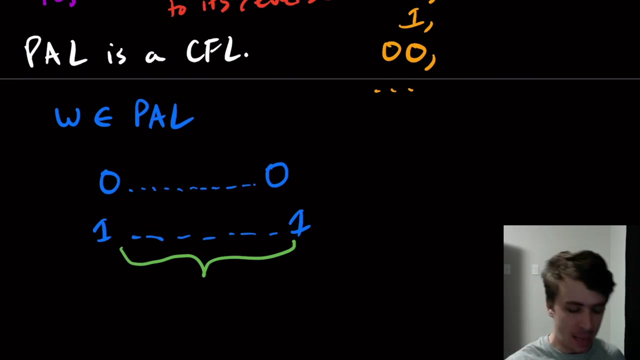 smaller problem, then how can you solve the bigger string? Well, what is happening in the middle? Well, because the string is the same backwards and forwards, then that means that the stuff in between the zeros or between the ones, that must also be a palindrome, because the string is exactly. 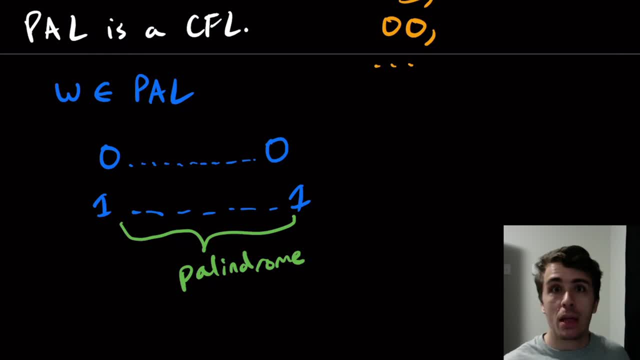 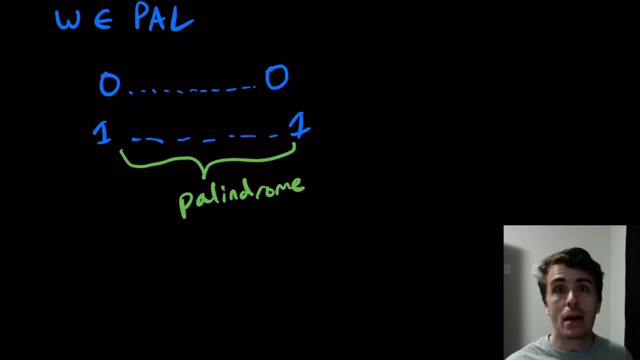 the same backwards and forwards. So this is a prime example of using the definition of the language in a recursive way. So how can we actually make a grammar for this? Well, let's just take this into account: In every grammar, even in context-free grammar, we must have a start variable somewhere. 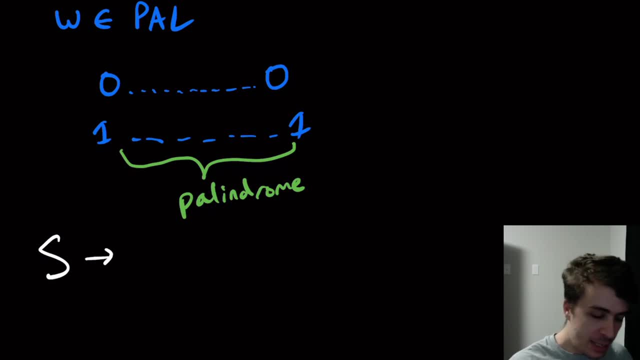 so let's call it s, So s is going to make. well, what are the things it can make? It either can make the empty string, Because the empty string is a palindrome by definition, Or so this is you can actually. 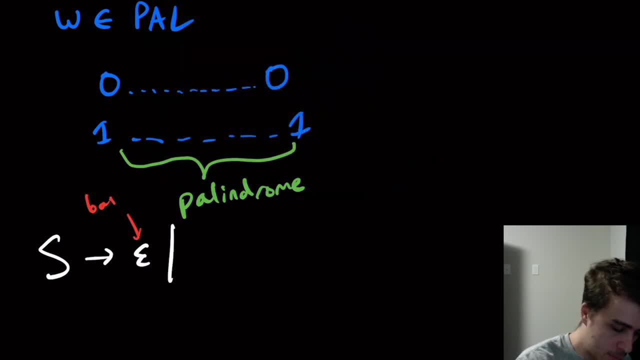 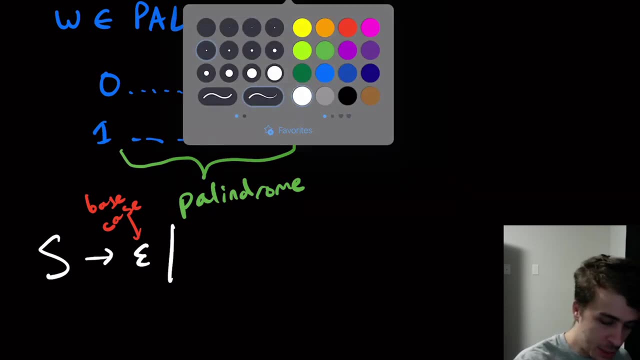 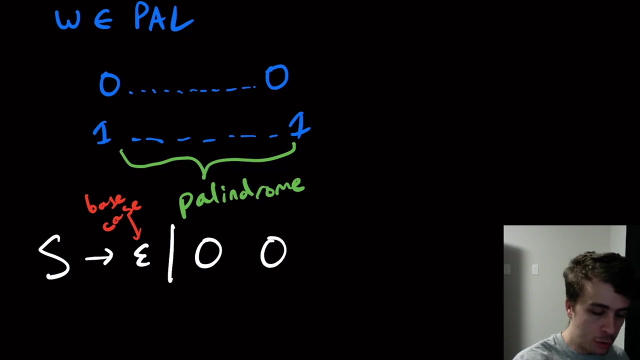 think of this as being a base case. So a base case. And then what are the inductive cases? So the inductive cases are when you have the zeros on the end And then we're going to assume by recursion that s could make all the palindromes. 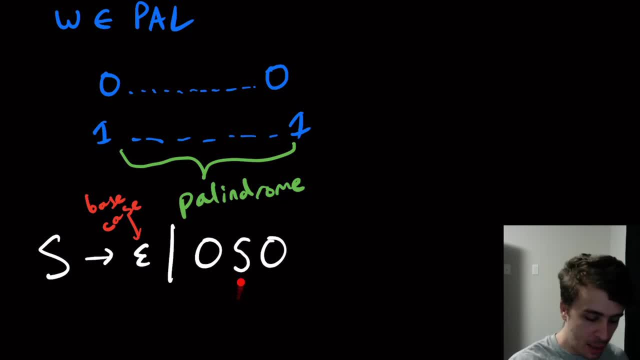 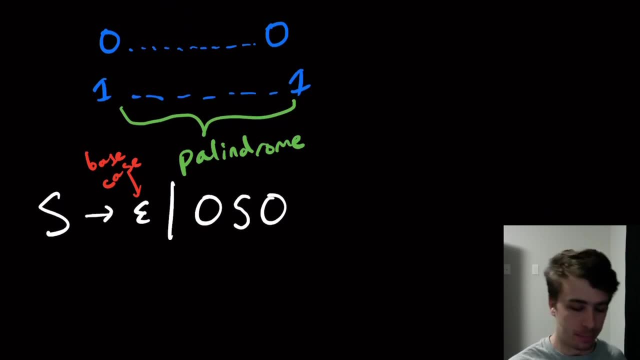 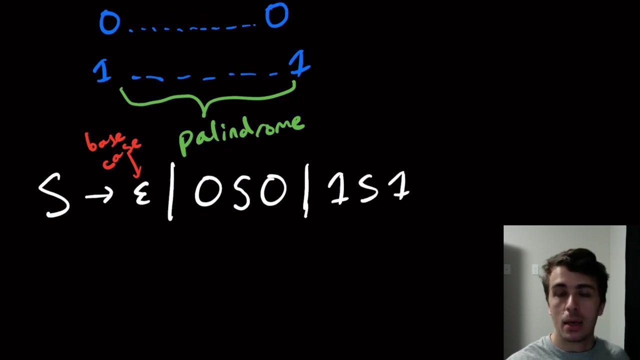 So by putting an s right here, that's saying, assume that I can make a palindrome, then that means I'm allowed to put zeros on either side, and that's also a palindrome, And the same logic applies if I want to do this with the ones. This is almost correct, though, But we notice that. 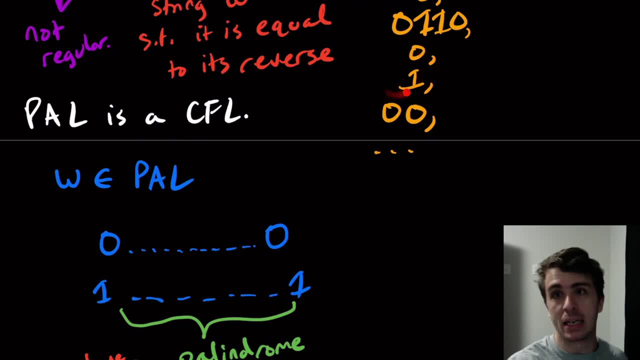 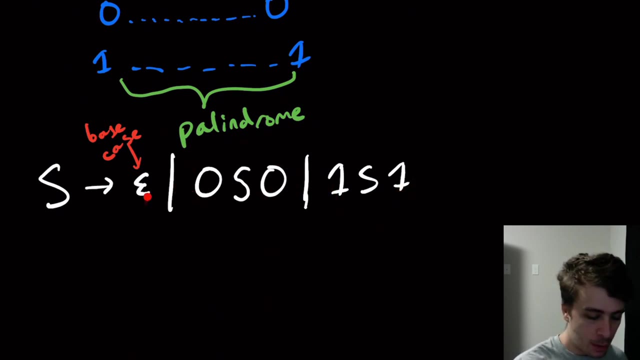 we have the individual characters being zeros and ones, And in fact we could have any string of odd length, but we could also be a palindrome. So if you actually look at this, we always will generate two terminals in every row, or zero, which is in the case here. So then that means that whatever 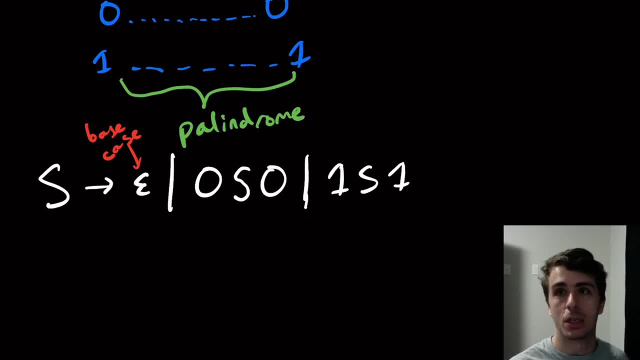 this makes is all the even length palindromes. So to get this to work with odd length, all we need to do is to handle the other two base cases, which are the individual characters. So we're going to do that. So these two right here are also base cases, And the ones here, these two, these are the 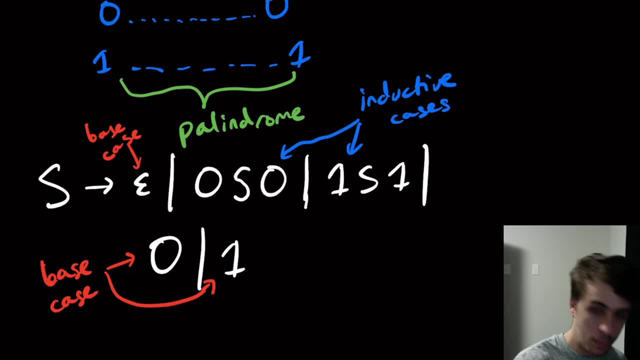 inductive cases. So this was a and you can actually prove via induction that this is correct because, apart from the middle, everything else has. there's an even number of characters Other than either the middle character or the middle character. there's an even number of characters. 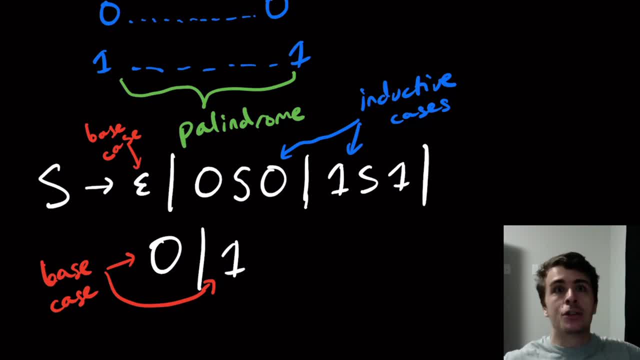 So everything else. there's an even number of characters, which means we apply these two rules over and over as needed. Then, if there are, if the string length we want is even, then we apply this rule, And if the string length is odd, we apply one of these two, whichever one is the one.